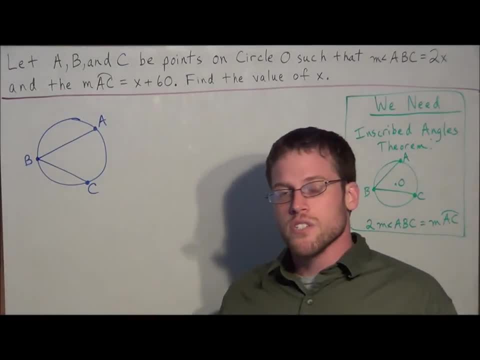 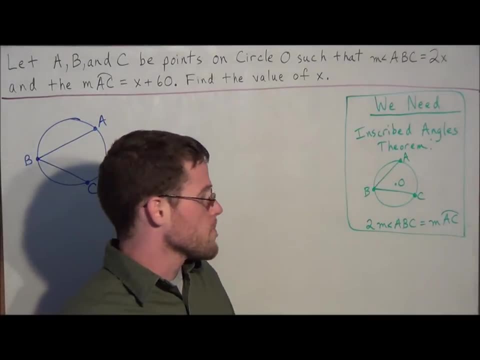 the measure of arc. AC equals X plus 60. And using this information, we want to find the value of X. So to solve this problem, we're going to make use of the inscribed angles theorem. Now, this theorem could be a little bit confusing when there's letters involved. 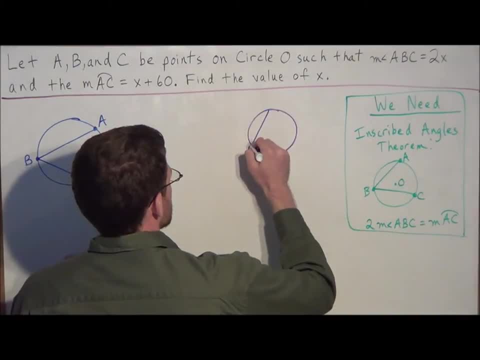 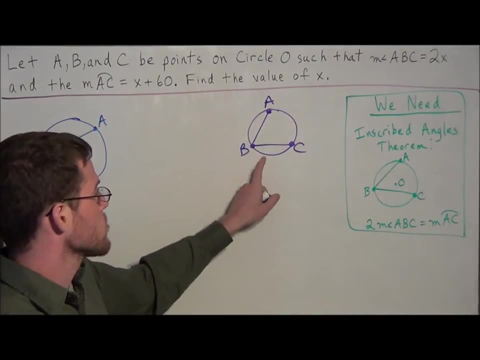 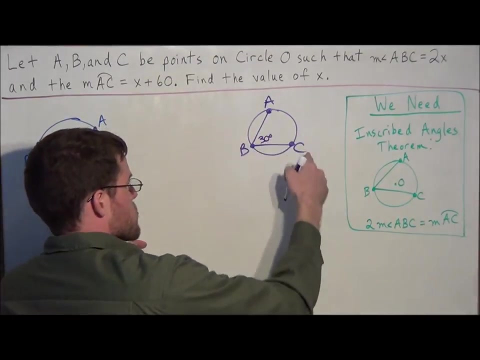 so just a quick explanation of what it is, using real numbers. If we're given an inscribed angle- and remember an inscribed angle is just an angle whose vertex is on the circumference of the circle, And let's say we're told that this is 30 degrees, then the measure of the 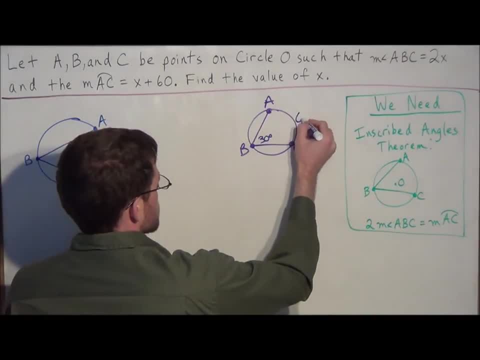 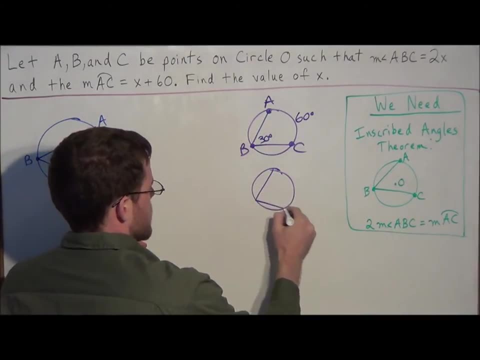 arc is twice the measure of the inscribed angle, so this would be 60 degrees, which is just 30 degrees times 2.. So let's say we were given that this is 100 degrees and now these aren't drawn to. 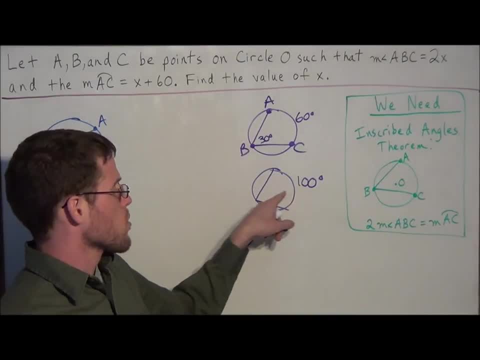 scale, but to find the measure of the inscribed angle, if we're working backwards, we would just divide 100 by 2, and get 50. And notice, 50 times 2 gives us 100, so these satisfy the rule. So we're just: we double the inscribed angle to get to the measure of the arc and 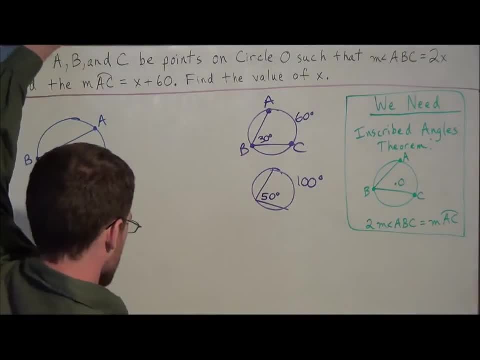 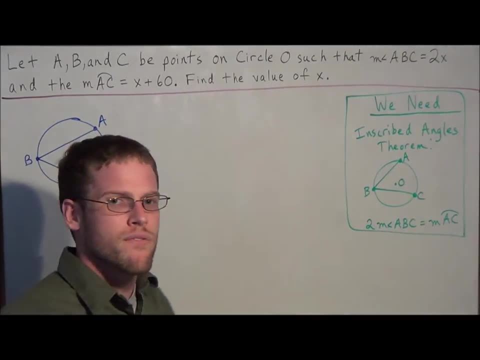 if we're going backwards, we divide by 2.. But, as you're going to see, multiplying by 2 is usually easier because when you're dividing by 2.- Especially when there's algebra involved, you have to take the half or divide an algebraic. 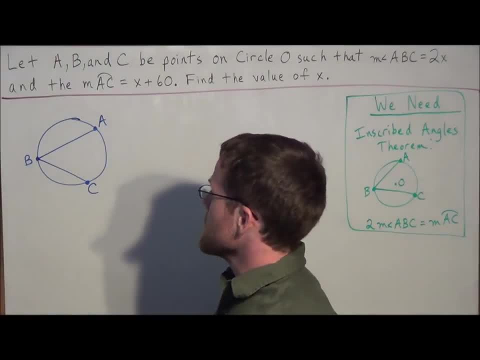 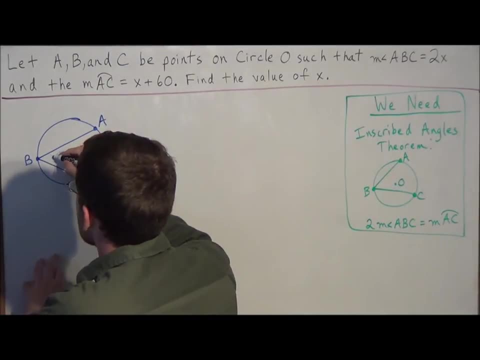 expression by 2, that could get a little tricky, so doubling is a little bit easier. So the first thing we should do is just label everything that was given to us. The measure of angle ABC is equal to 2x, and the measure of arc, AC, is equal to x plus 60. And if we 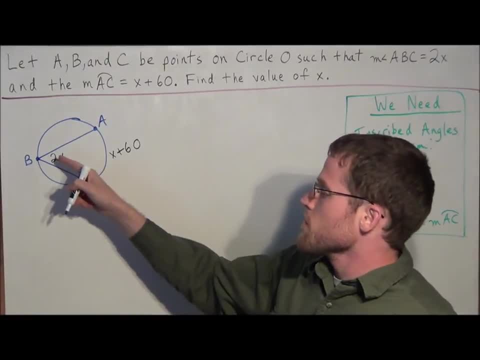 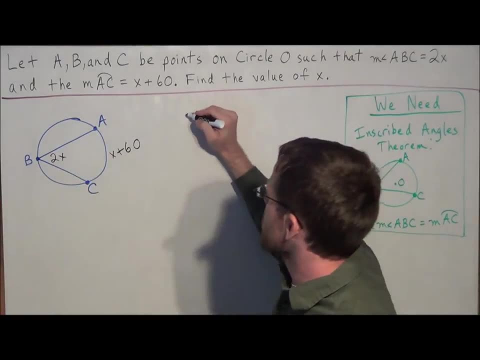 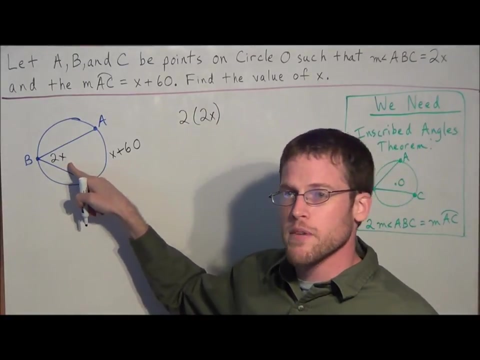 follow this theorem. we said that the measure of the inscribed angle is half the measure of the arc. So what we want to do is we're going to double the inscribed angle. So we're going to multiply 2x by 2, because we said twice the measure of the inscribed angle. 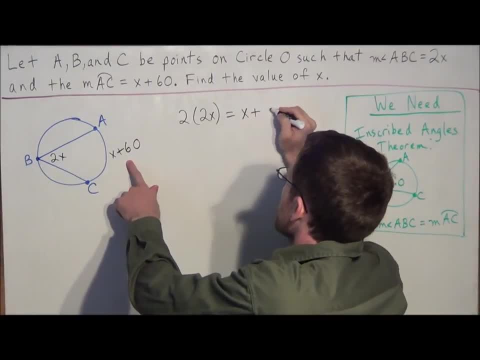 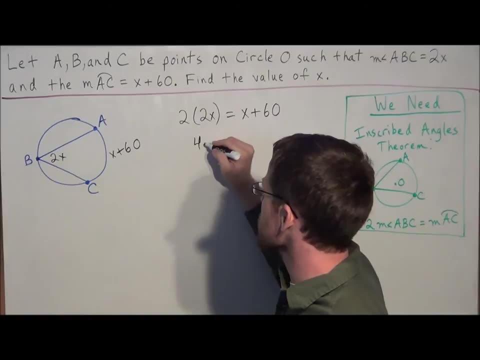 equals the measure of the arc, which in this case is x plus 60. So all we need to do at this step is just simplify the algebra. we're doing 2 times 2x is 4x, 4x equals x plus 60. So to solve, we're going to subtract x from both sides.